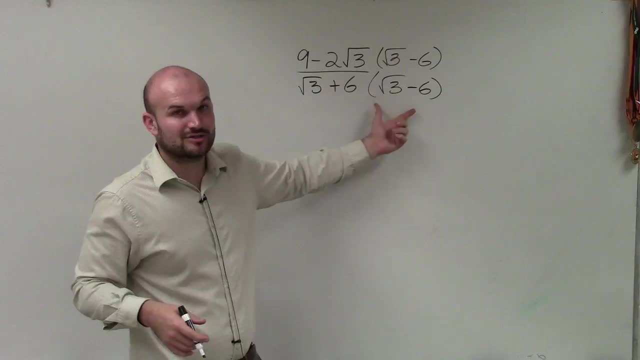 can get rid of our square root and our middle terms that we'd multiply by, add up to 0.. Now it's also important when we multiply by our conjugate, we multiply the denominator and the numerator the same. that's going to produce an equivalent fraction, which is not going. 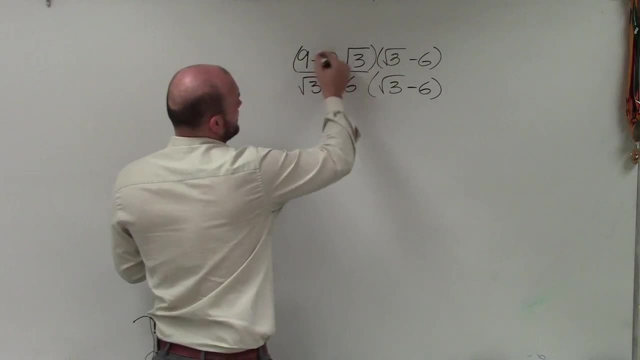 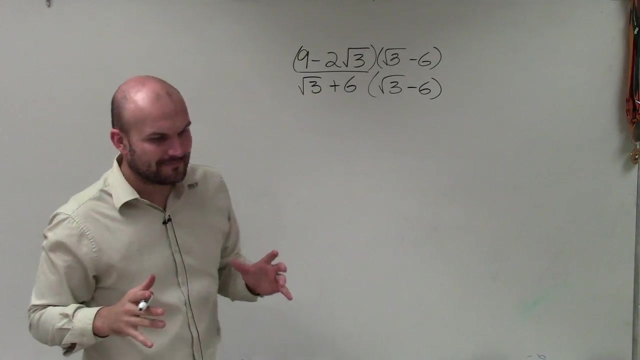 to change our answer, Alright. so really the hard part here is going to be foiling our numerator, Because our denominator is just a difference of two squares, which we understand. that I guess I can show it either way, But let's just kind of go through it again. So to multiply: 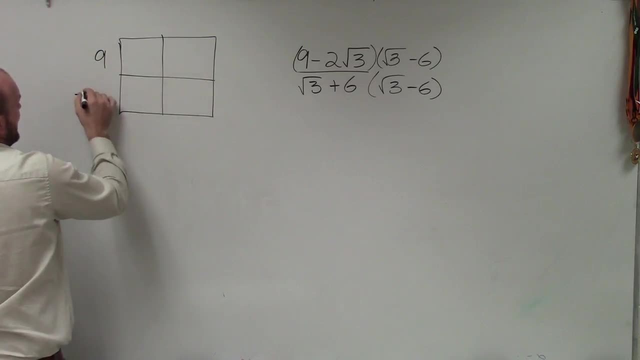 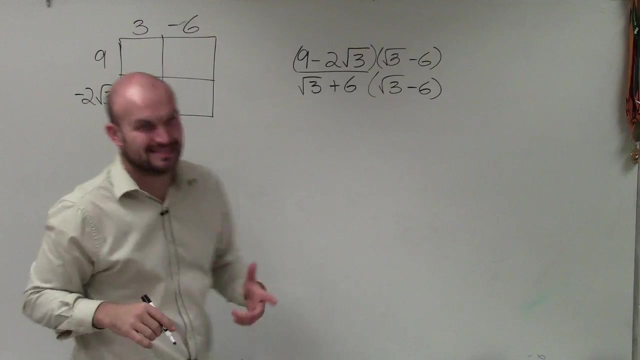 these. I think the easiest way that I like to do it is just to use a box, And I like using the box method because what it does is it allows me to kind of organize my multiplication very easily. Alright, so when you go ahead and go through this, I do 9 times 3, which 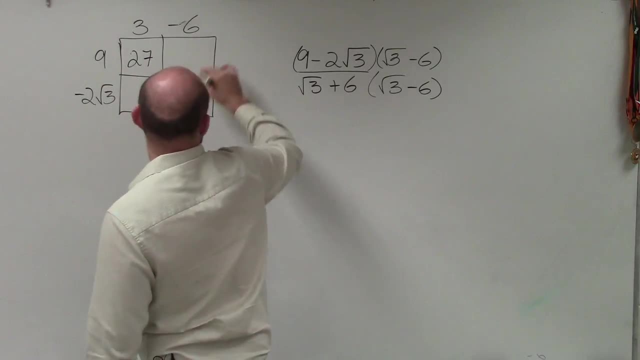 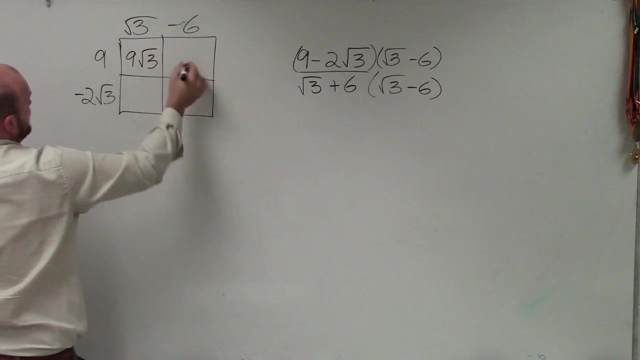 is 27.. 9 times 6,. oh wait, that's, that's 27.. Alright, so when you go ahead and go through this, you see the denominator of 4 times the square root of 3.. Alright, so it can pull. 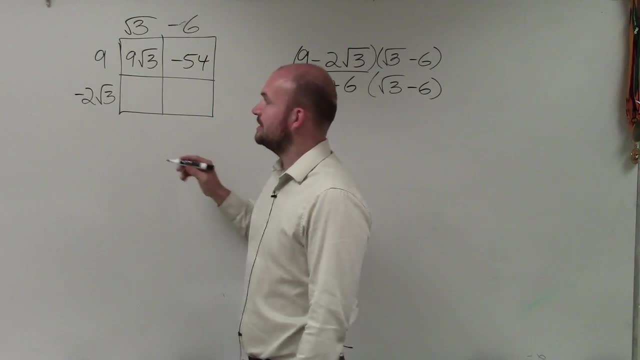 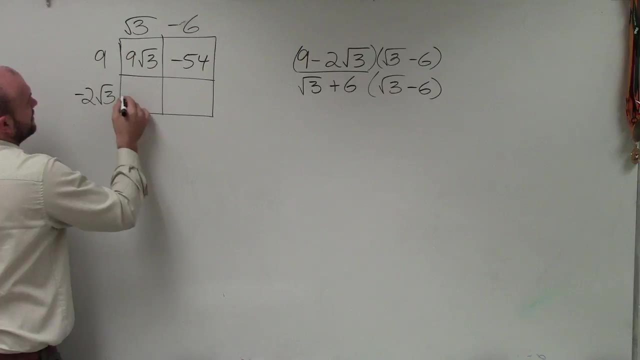 out the equation. So what's going to happen right now, if I go through this, is I'll just again see how I'm multiplying mu, because right afterwards, what I'm getting to find out is then what I could do is I'm going to sum this up, by the way, by leaving whatever. 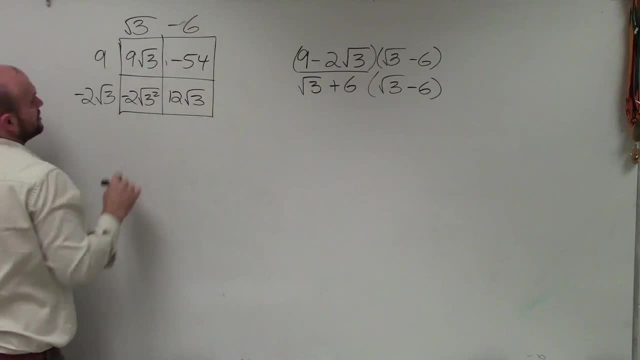 I need here right When you go to find it, what are you going to find? You're going to solve this by pushing the little under here, sort of switchion paper, and that leaves a little of the work out for you, Not that you just follow through over and over again, or? 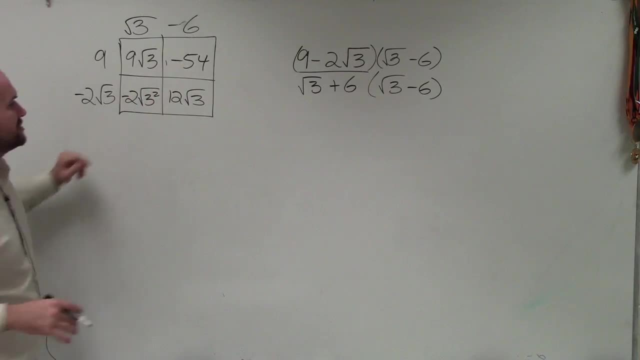 exactly like I was. Yeah, so faster, All right. so say, m of w needed three. okay, Well, but m of m of W had a variable and you're looking for some other variable here. So if you to 3, square root of 3 squared is just going to be 3, right. 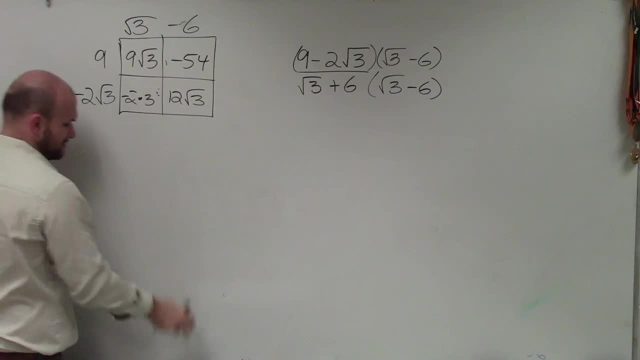 Square root of 3 squared is just 3.. So therefore I have negative 2 times 3,, which now gives me 6, negative 6.. All right, so now we can see. the nice thing about this is we can organize them. 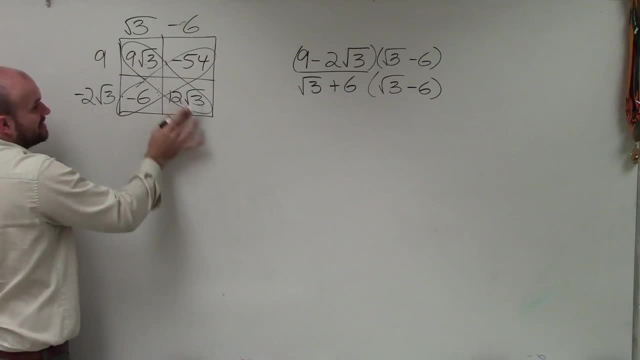 These have the same number under the radical sign. Our radicands are the same, so we can combine them. And these are both numbers, so we can combine them. So therefore I have negative 60 plus 21,, square root of 3..